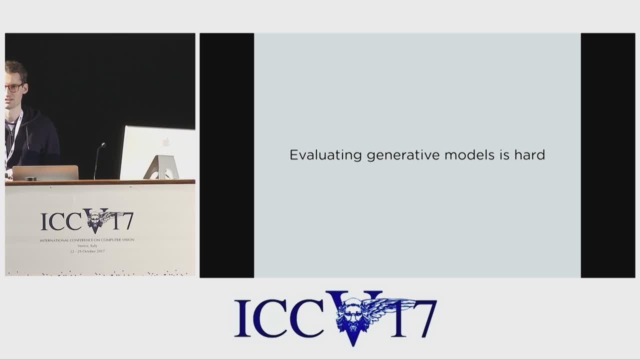 It's not just, you know, computationally difficult or technically challenging, But we don't, presumably we don't even know what should be evaluated. But I actually no longer believe that's true. Instead, I will try to convince you. 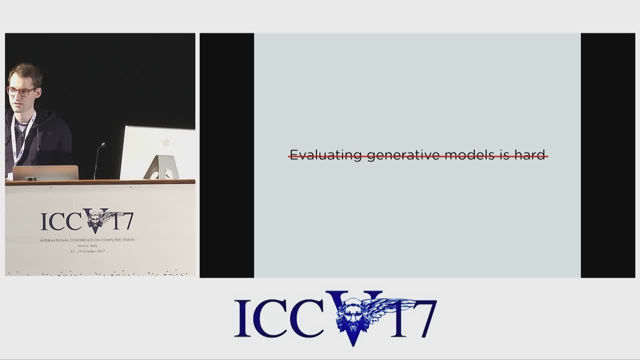 That if you just think about why you are training a generative model in the first place, what is the problem that you're trying to solve, And you keep asking why until you reach one or more clearly defined applications, then typically it becomes pretty clear what a good evaluation looks like. 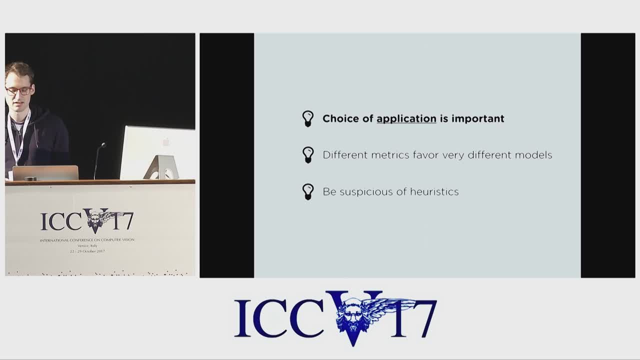 So one of the take home messages which I will try to convey is that thinking about applications will make your life much easier, even if you are not actually that interested in the application itself but are more interested in developing it. And also if you think about your application and the applications themselves rather than thinking about different ways of developing methods. thinking about applications will make it easier for you to come up with a meaningful evaluation. 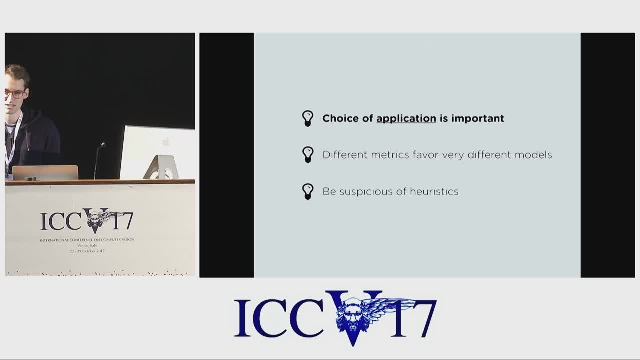 And it is also necessary to think about applications because, as we will see, different application have extremely different requirements. So I used to have this dream that you could completely separate probabilistic modeling, or generative modeling, from applications, That you could first, for example, model the distribution of natural images. well, in some general sense. 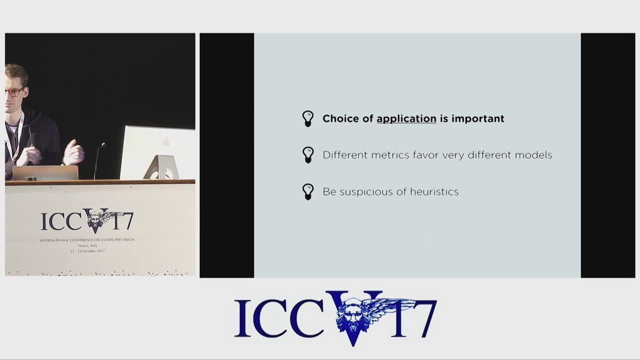 And then I would automatically turn to play the role of the generative model. I used to have this dream that you could completely separate probabilistic modeling or generative modeling from applications. do well in all kinds of applications, like denoising, compression, representation, learning. 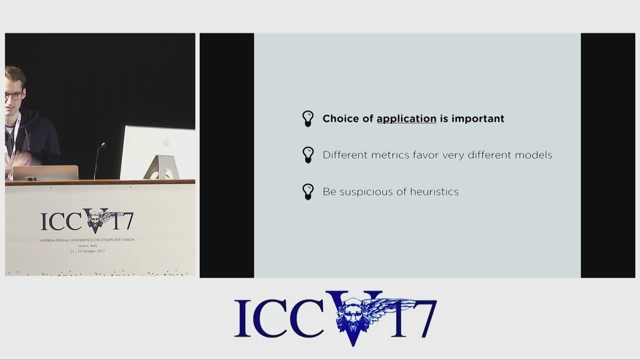 synthesis and so on, And this kind of separation can work well in low dimensional, simple problems, but, as we will see, it can also completely fail in high dimensional, hard problems. So at least when it comes to evaluation, we really have to know what we want and choose. 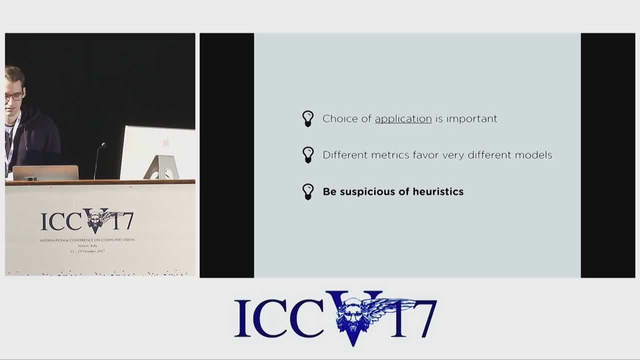 the right tool for the job. And this also brings me to my third take home message, which I will try to convey, which is be suspicious of heuristics. I think because we like the separation between generative modelling and applications, we sometimes try to avoid applications and instead try to come up with some general heuristic. 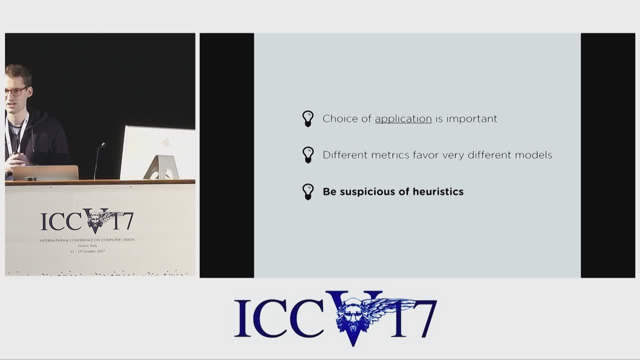 that tries to capture the overall performance of a generative model, And this is problematic for several reasons. One I already mentioned: there really is no single metric which can capture the performance of a generative model because different applications behave so differently. And the other is that these heuristics are often based on intuitions which hold in low. 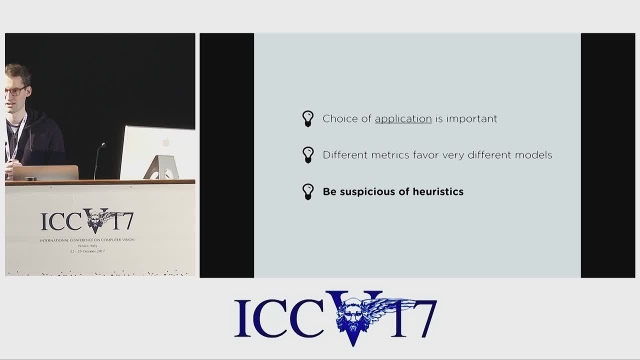 dimensions but can fail in high dimensions, And this means these heuristics are often. it's often possible to cheat these heuristics, as we will see. Okay, to start, let's take a look at some applications. So the first thing I want to do is to show you some examples of heuristics. 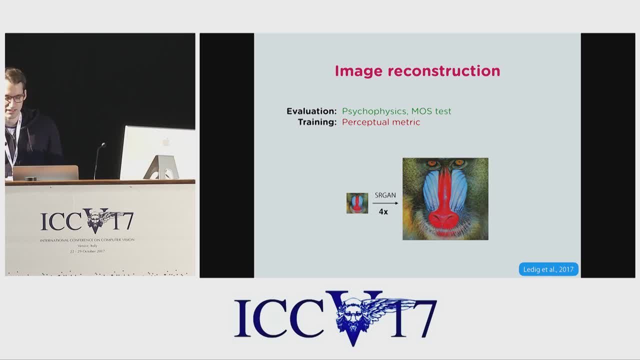 Let's take a look at some applications, Some example applications, and let's start with something that GANs are really good at, which is generating realistic images. But there's only a few applications where you really want to generate images from scratch, out of thin air. 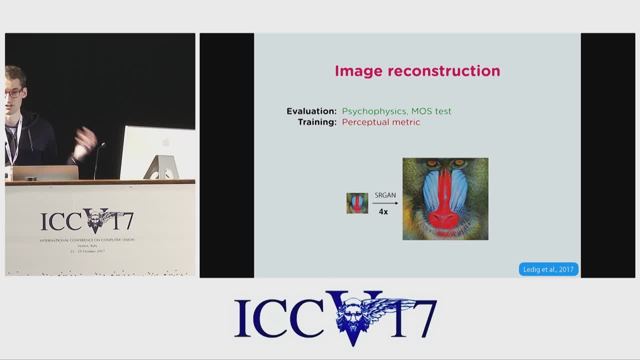 Typically, you have some kind of information on which you want to condition your samples on. For example, you want to generate some images from a text description, or you want to change the style of an image, Or, in the case of SRGAN, here you want to generate a high resolution image conditioned. 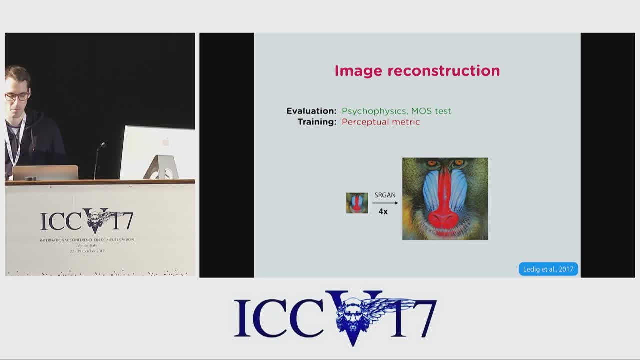 on a low resolution version of that image, And it's pretty clear what we want from that model. We want it to generate images which, to us as humans, look as similar as possible to the original image. For training, that would mean optimizing a perceptual metric which agrees with how we 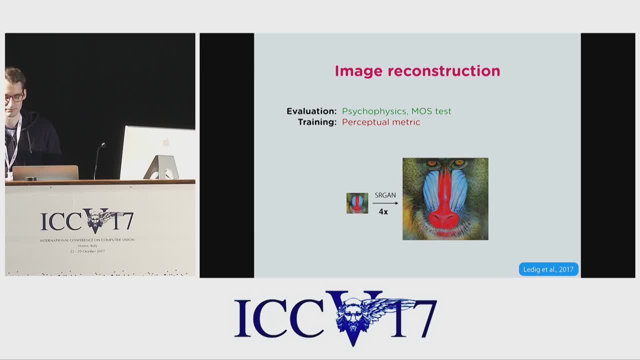 how our brain perceives differences between images And of course, that's really hard because we don't have a good perceptual metric. it's an unsolved problem, Which is why we're using GANs and other tricks, But for evaluation we really don't have to be able to optimize this perceptual metric. 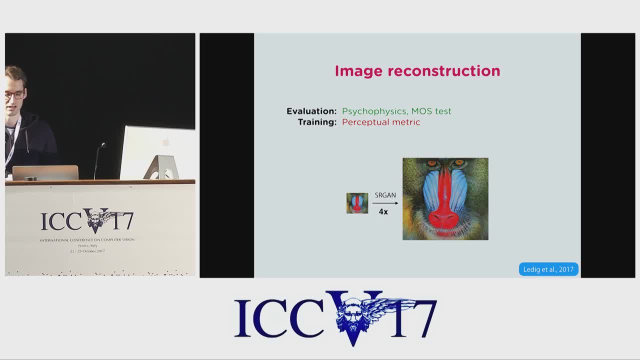 all we have to do is be able to query it, And that we can do with psychophysics, which is basically, you know, putting people into a kind of controlled condition and asking them questions, Or, even simpler, a mean opinion score test, where you simply show the reconstructions. 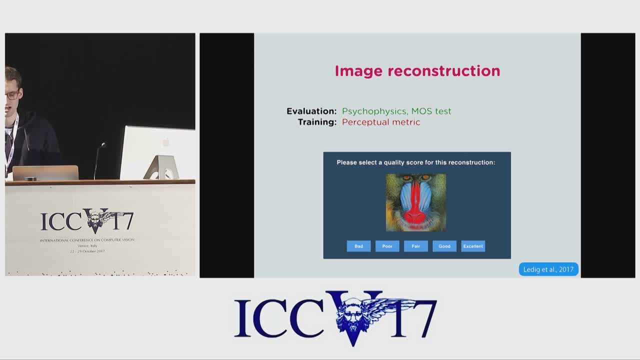 to people and ask them, you know, on a scale from one to five, how do you rate this reconstruction? And, in the case of SRGAN, using the right evaluation really paid off If you use something like PSNR or Structured Similarity Index to evaluate the reconstructions? 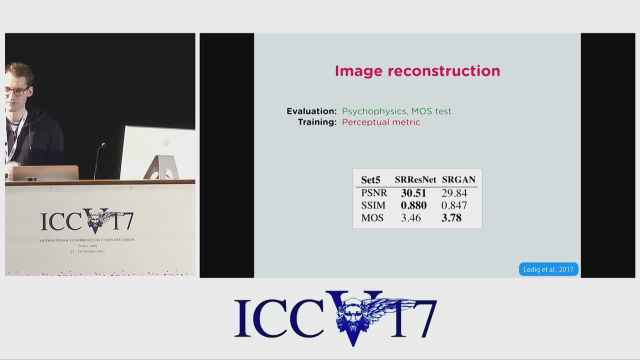 you'll find that an SRSnet optimized for mean squared error outperforms an SRGAN, even though if you ask people in a mean opinion score test, you'll find that an SRGAN actually outperforms an SRSnet by a large margin. 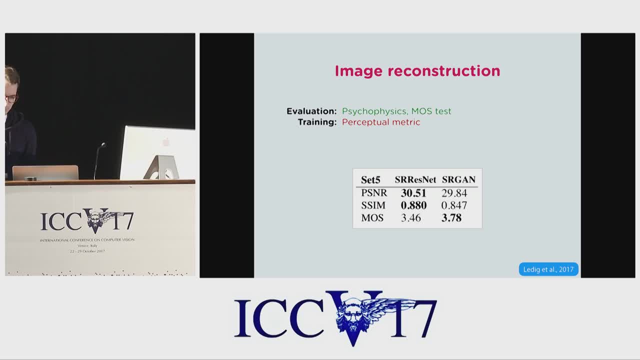 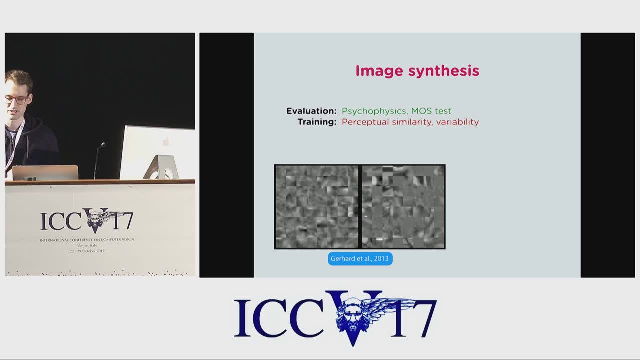 Thank you, Thank you. So I just want to mention one other interesting psychophysics approach which has some advantages over MOS tests and might be particularly useful in the rare cases where you actually do want to generate images from scratch, For example in texture synthesis, which is sometimes used in games. you want the outputs. 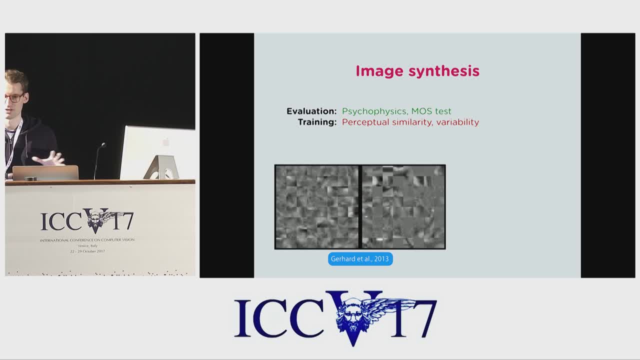 to be perceptually similar in some sense, at some level, to the training data. but you also want some variability. You want the output to have some entry. So in this psychophysical paradigm, what you do is you sample images from your model or you sample patches from your model and you arrange them in a kind of texture so that 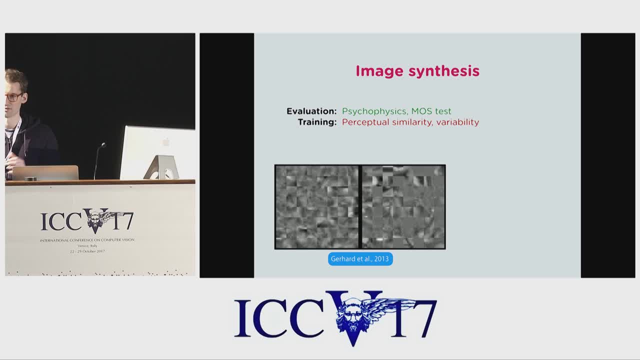 you can see many samples at once and judge the distribution of variability of your samples. You do that for samples from your model and you do that for test images, And then you ask observers which of these two textures comes from the real data and which one is fake. 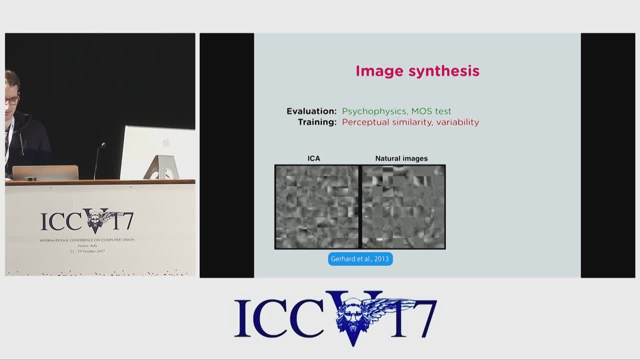 In this case we have samples from ICA on the left and real images on the right And, of course, if the model does well, it will be very hard to distinguish the textures and if the model does poorly, it will be easier to distinguish the two textures. 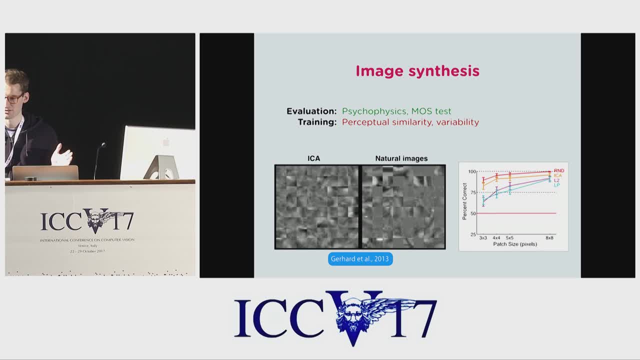 And one nice thing about this approach is also that now we can change the size of these patches and get a sense for the scale at which your model performs well and the scale at which your model performs poorly. So on the right-hand side here we have, on the x-axis, the patch size of the sample textures. 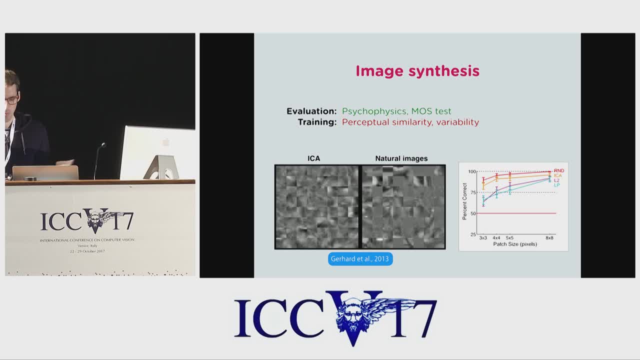 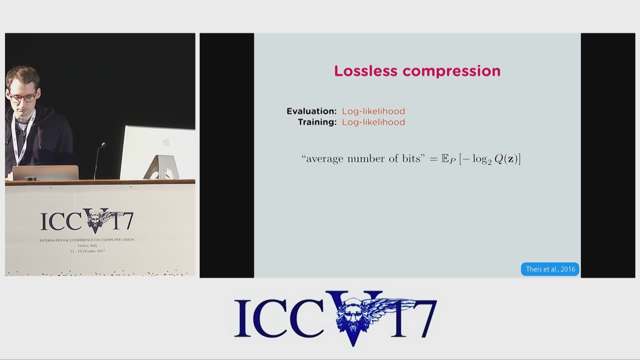 On the y-axis we have the performance of the observers and you can see that as the patch size increases, people find it easier to detect the real images and you can imagine how a better model will push these curves down. So a completely different application actually is lossless compression. 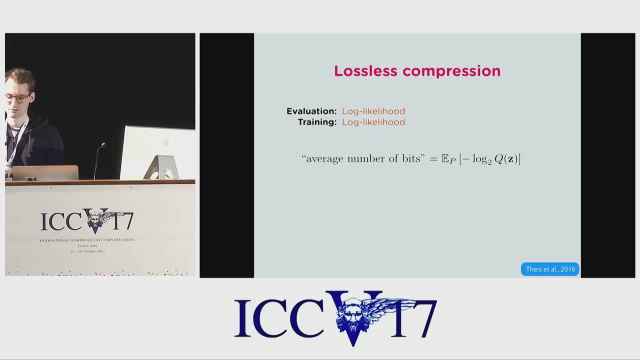 If you use something like a range code, you can see that the lossless compression is very important. If you use a large encoder to compress your data, to encode it into bits, the average number of bits that you will get is roughly the expected negative log likelihood that you assign to. 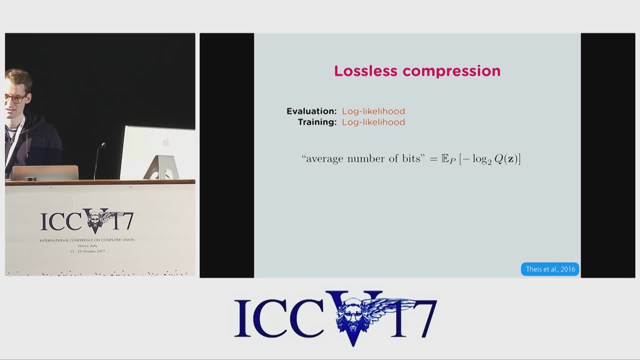 that data. That's one caveat, and that is that this only works for discrete data. For continuous data, this is not true, and this has to do with differential entropy having some problems. So if you wanted to encode a continuous random variable to arbitrary precision, you would. 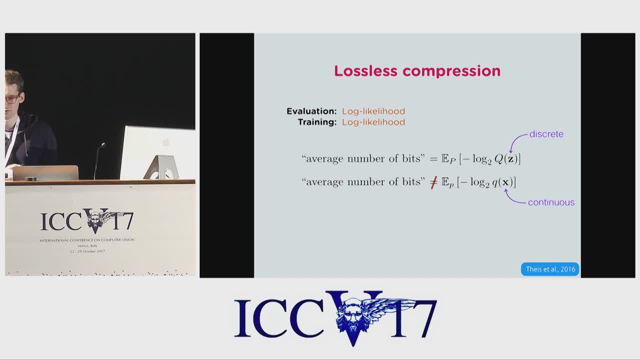 require an infinite number of bits, and so the negative log likelihood for densities does actually not represent information. But luckily there's also an easy fix. I'm not going to go into details here, but basically all you have to do to fix this is. 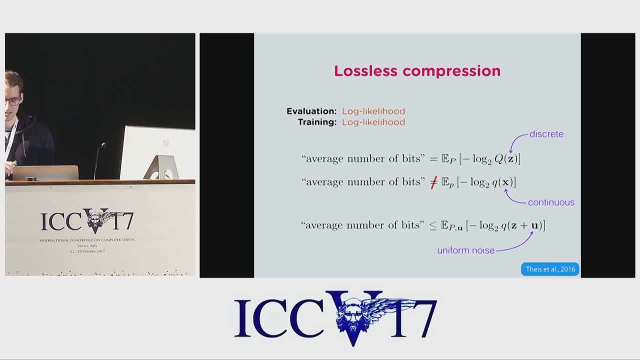 to add uniform noise to your integer data and you'll get a meaningful quantity to evaluate, because this quantity represents an upper bound on the number of bits required. So if you want to encode a continuous random variable to arbitrary precision, you would require an infinite number of bits, and so the negative log likelihood for densities does. 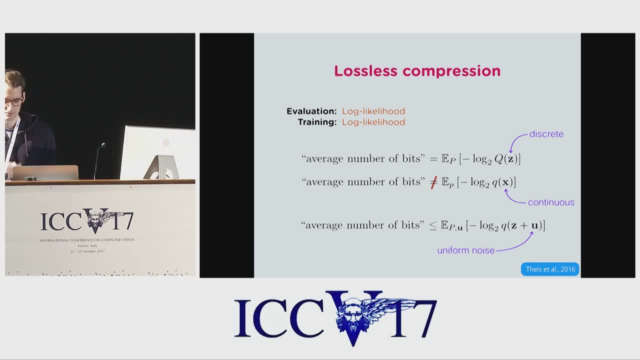 actually not represent information And you also need an infinite number of bits to compress this integer data. Unfortunately, for GANs and other decoder-based generative models, evaluating likelihood can be quite difficult. It's nevertheless possible. This paper from Toronto shows that you can use annealed importance sampling to evaluate. 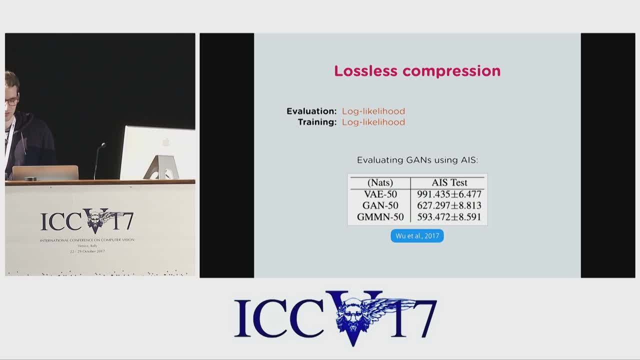 decoder-based models and, unsurprisingly, you find that models optimized for log likelihood, such as variation autoencoders, outperform models which aren't optimized for log likelihood, such as GANs. But I would also argue that if it's that difficult to evaluate the log-likelihood of your model, 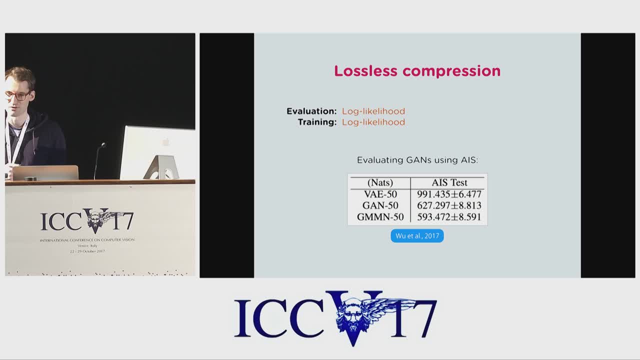 you probably weren't thinking about using this for compression anyway, So there's probably a better way to evaluate your general model. And vice versa. if you were thinking about using this for compression, you probably designed it in a way that you can evaluate the log-likelihood easily. 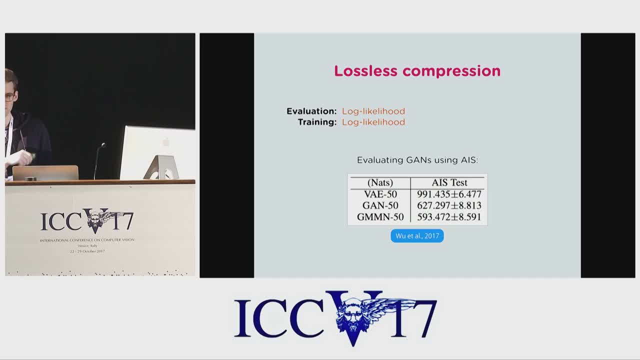 So I would argue that in most cases where you want to evaluate log-likelihood, evaluating log-likelihood is also easy. Finally, unsupervised learning is probably the best example where training is extremely difficult, but evaluation can be easy Because we typically have some downstream tasks in mind, or at least we should have. 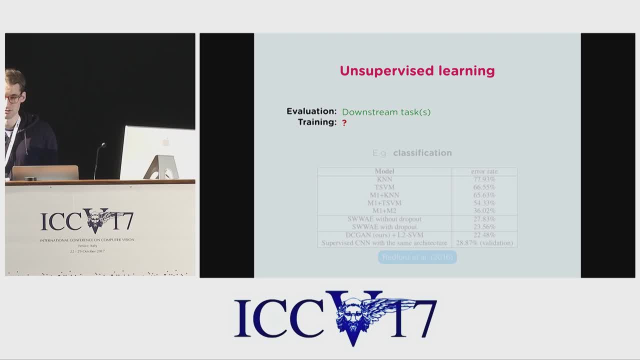 some downstream tasks in mind when doing unsupervised learning, For example, when trying to learn representations for classification. a good way to evaluate your representation is to evaluate your representation, And a good example of this very common practice is the DC GAN paper. 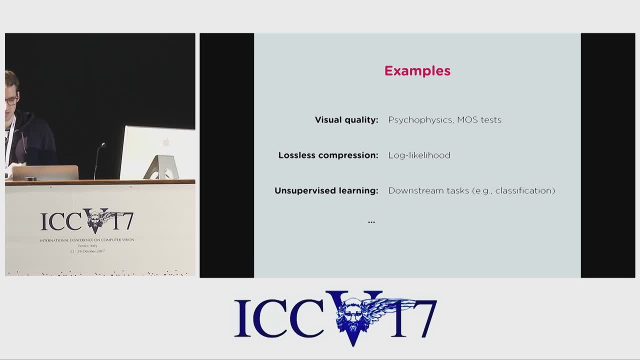 So, to summarize this part, we've looked at a couple of examples of how you can evaluate your generative models for different applications And, in particular, if you're interested in the visual quality of your reconstructions or samples, your evaluation should probably involve some people. 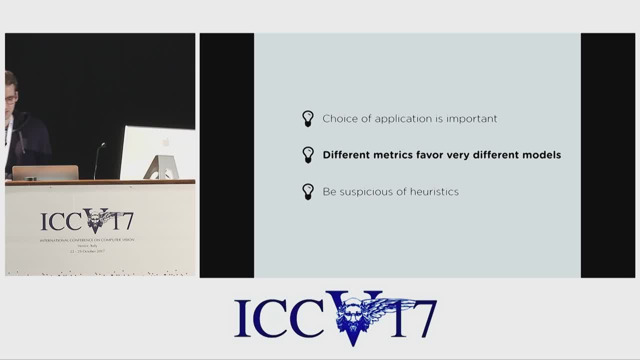 Now let's take a look at how differently different metrics and applications can behave, to see that it really matters which of these applications you use to evaluate your generative model. So here's a little toy example where we have a histogram of two-dimensional data in the 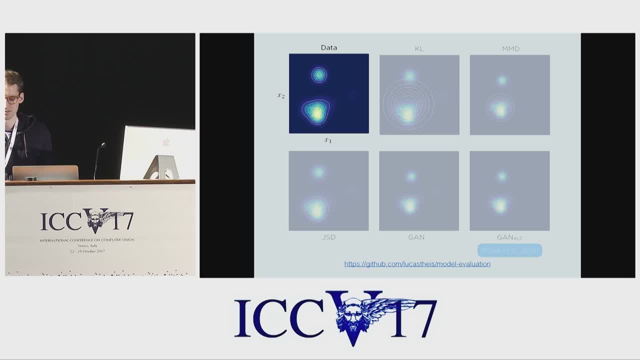 top-left corner And we're going to fit an isotropic Gaussian value. So we must first get rid of the two-dimensional data in the top-left corner to this data. We use this simple model because we're interested in this regime where there's 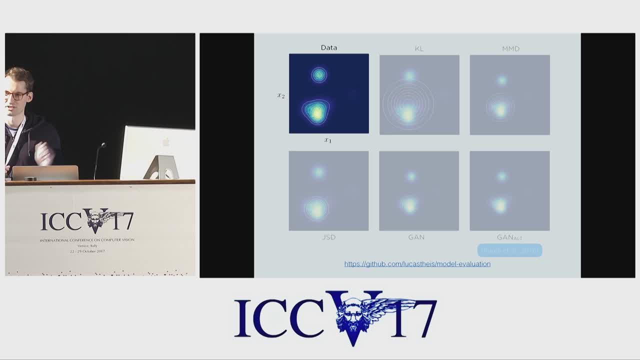 a mismatch between your model and your data because you know, for the kind of interesting problems, high dimensional, difficult problems, there is going to be a mismatch between your model and your data. So if we fit this model with respect to KL divergence or equivalently log, 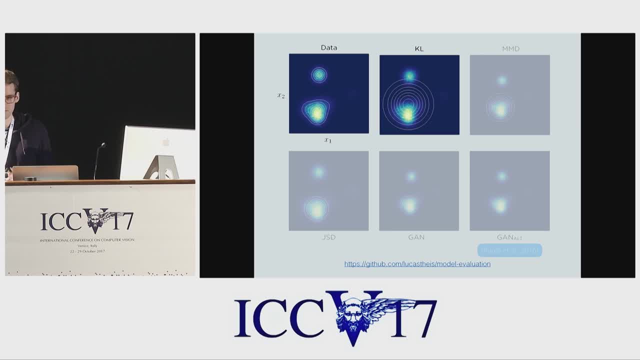 likelihood we would get a fit like this. Our Gaussian tries to assign at least some probability mass to all the data points, but this of course comes at the cost of assigning some probability mass to regions which aren't data. So when you sample from this model, you would 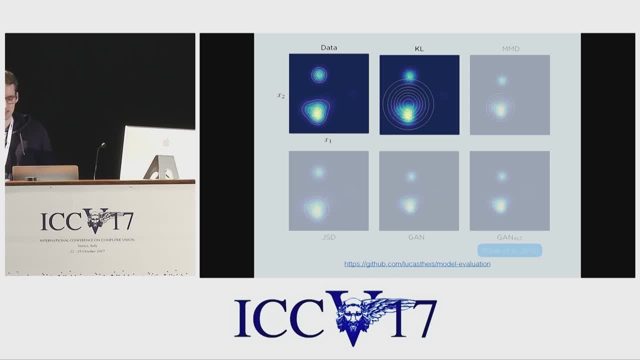 get a lot of data points which don't look like the data, but on the other hand, this fit would be optimal for compression. If you use maximum mean discrepancy to fit the same model, you would get a much tighter fit to one of the modes. If you use Gans and Chen divergence, you would get 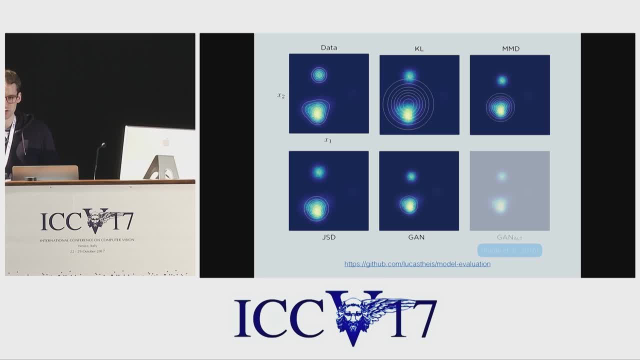 an even tighter fit and, of course, at least in theory, we could use Gans to approximate this Gans and Chen divergence, although of course, in practice, the fit that you get might be very far from Gans and Chen divergence and depends heavily on the discriminator that you use. In practice, we also often use this. 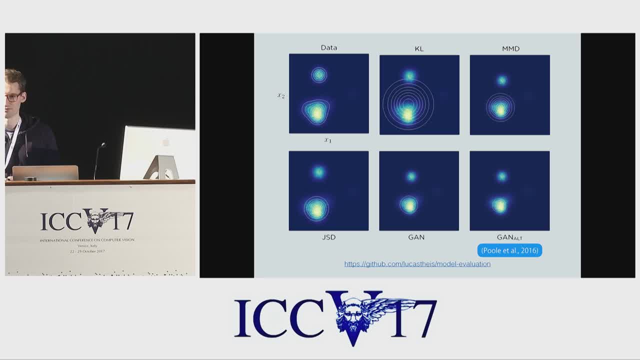 trick To get better gradient information for the generator, and Ben Poole discovered that if you use that trick, you get even more extreme zero avoiding behavior, and we also find this in this toy example. we get an even tighter fit to one of the modes And this is great if you want to generate realistic 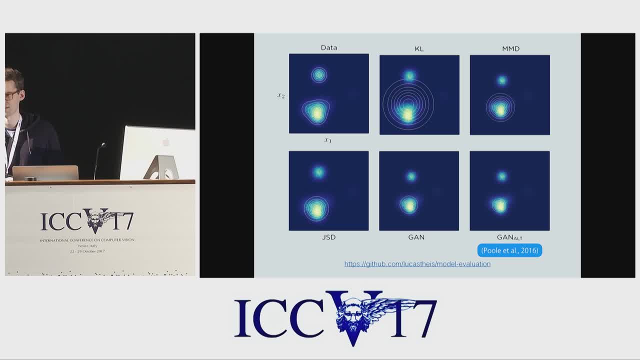 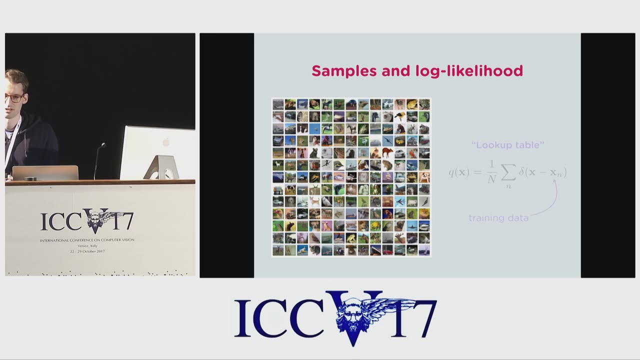 images, because now all your data points will look realistic. but of course, this comes at the cost of completely ignoring one of the modes, and this would be terrible for compression. Now let's take a look at a closer look at two commonly used methods or criteria for evaluation. 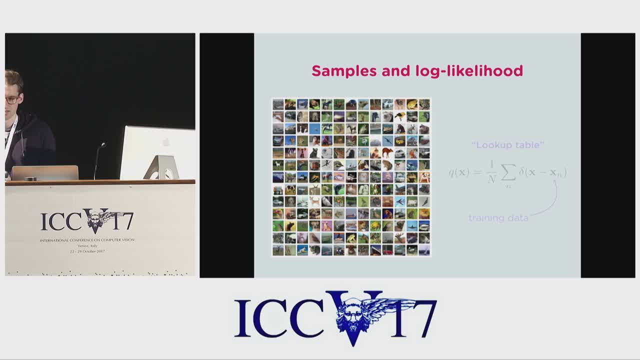 which is the visual quality of samples and the log likelihood of a model. Of course, we all know that getting good samples at the cost of you know, while also having a poor log likelihood, is extremely easy. All you have to do is you have to overfit to your training data. or, even simpler, you. 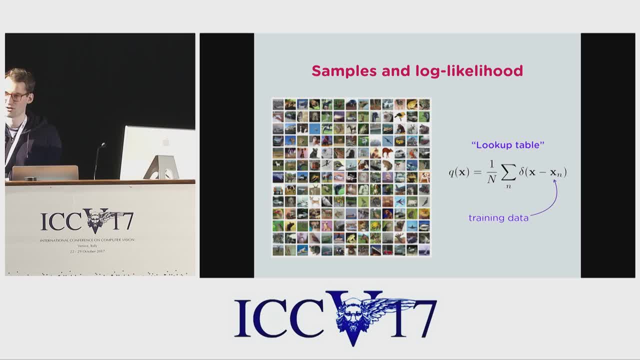 can just basically create a lookup table, and then you can just create a lookup table, and then you can create a lookup table which stores all your training images, and when you sample images, you just sample from this lookup table. this is the perfectly well-defined probabilistic model which 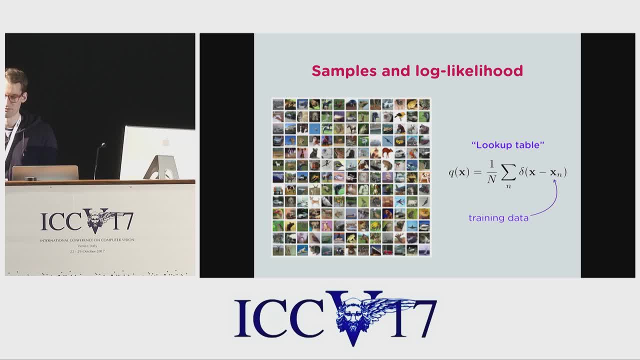 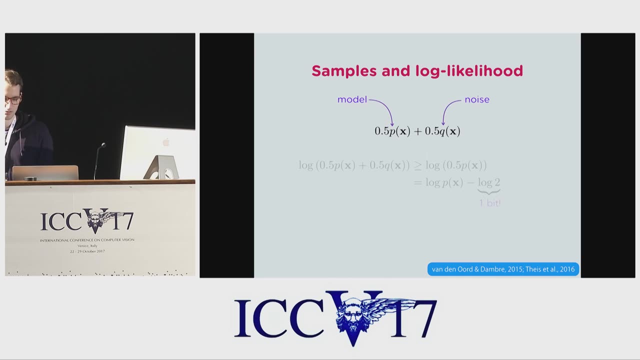 has an extremely poor log likelihood but perfectly fine images. What is maybe less obvious is that you can also have extremely good log likelihood and still create generate extremely poor samples. So to see this, what we do is we take our model with a, you know arbitrarily perfect log likelihood p, and we mix it with 50% noise. So now, 50% of the time we're not 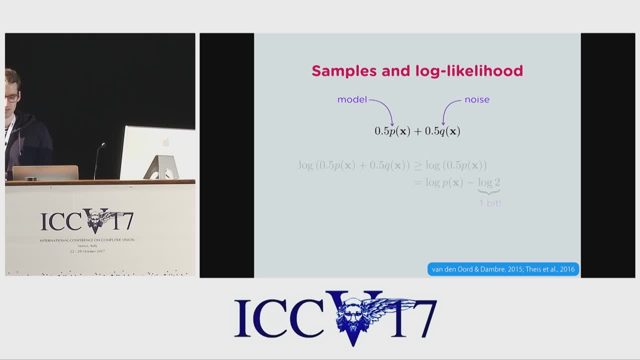 sampling from our model. we sample from a noise distribution which generates nonsensical images, But the log likelihood of this mixture model, as you can easily show, is at most only one bit worse than your original model p. And one bit is really nothing in high dimensions, where the difference between 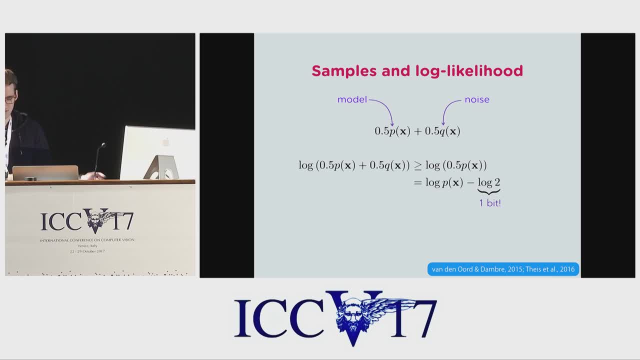 good and bad models are not as important. So we can go more extreme and mix in 99% noise. So now, almost all of all of the time we sample from this noise distribution and our log likelihood would be at most 4.61 nets worse. So your log likelihood would still be almost the same. 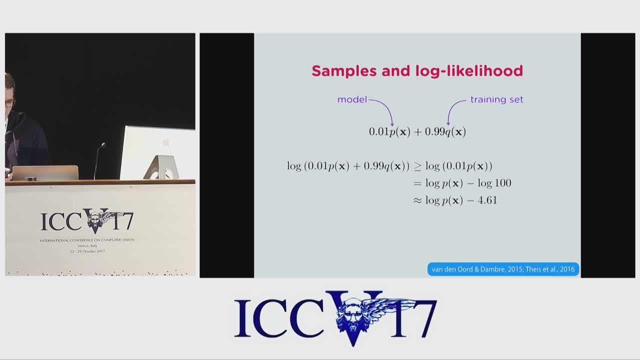 A note that we don't have to necessarily mix in noise Here. we can also sample from our lookup table and generate perfectly realistic images. So what this shows us is that you can have and mix and choose arbitrary sample quality with arbitrary log likelihood. So you shouldn't draw any conclusions about the log likelihood from the visual quality of your samples and you shouldn't draw any conclusions about the sample quality from your log likelihood. 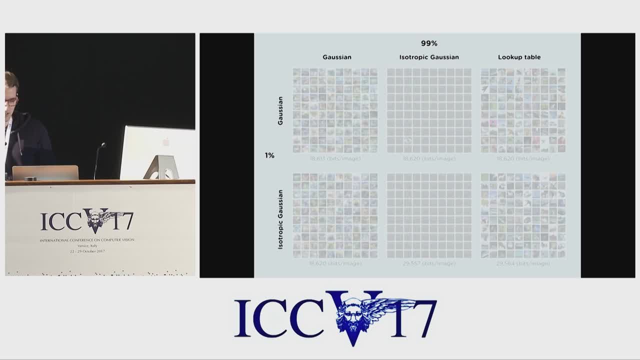 To visualize this a little bit more on a more interesting example, here we have models p in the rows, from which we sample 1% of the time, and we have other distributions, q, from which we sample 99% of the time in the different columns. 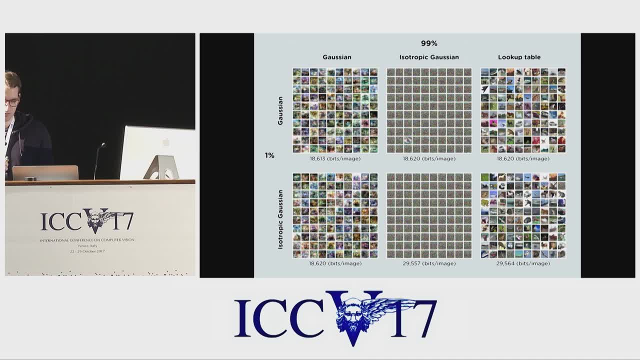 And then here I'm showing samples from the mixed term model, which are of course, dominated by the models in the different columns, and below the samples we have the compression performance of the mixed term model. Now, if we look at the first row, we see that you can have very different samples for almost 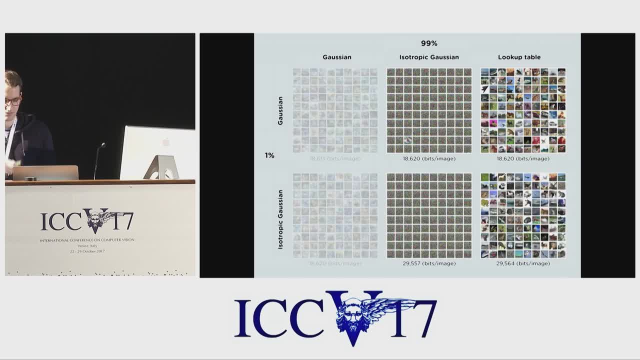 exactly the same compression performance And if you look at the last two columns, you see that you can have almost identical samples but completely different compressions. So again, this just means that you can't really draw any conclusions about compression performance from samples and vice versa. 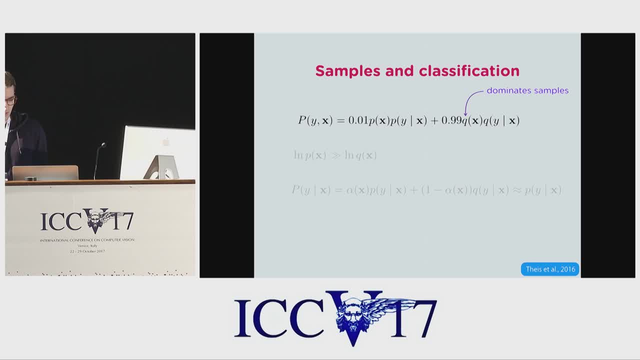 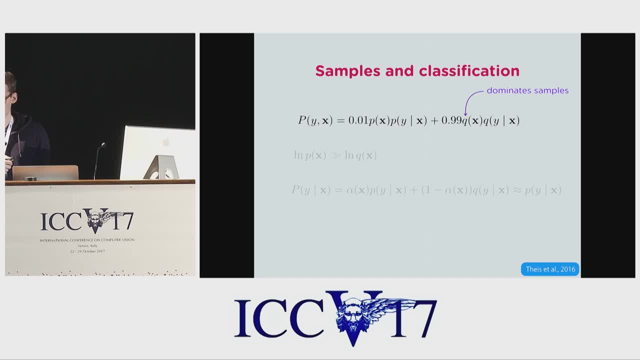 So ni example of this range expression can work just as favorably up against a class label. P and Q is associated, homologated as positive scenarios, and rapidly וה際 into three factors. So the first one is: if we com重 mx, You can observe: 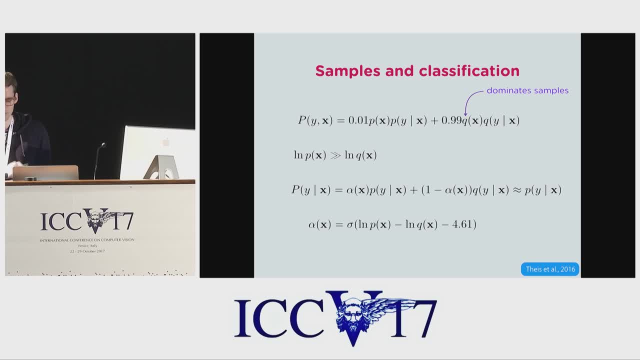 that the latter is always lipstick inclusive, so we can't practice that. by having two aberrations, You can show that the latter, in this case, will be dominated by P, Because the posterior is again classifier, which depends on the log likelihoods of the two models. So again, 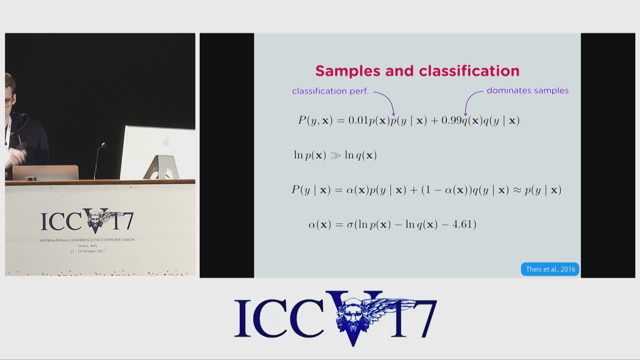 here the sample performance will be dominated by Q and the classification performance will be dominated by P. So again you have the situation where you can mix and choose arbitrary classification performance with arbitrary samples. So perhaps one way of thinking about this is as this kind of orthogonal 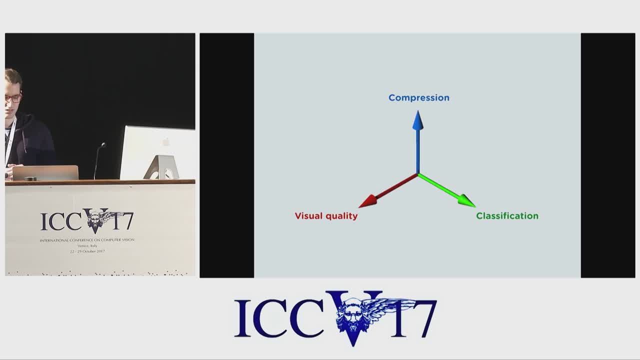 features of your generative model, where you can change the compression performance, the classification performance or the visual quality of your model without affecting the other two dimensions. So, finally, let's take a look at some common heuristics which were used for evaluating generative 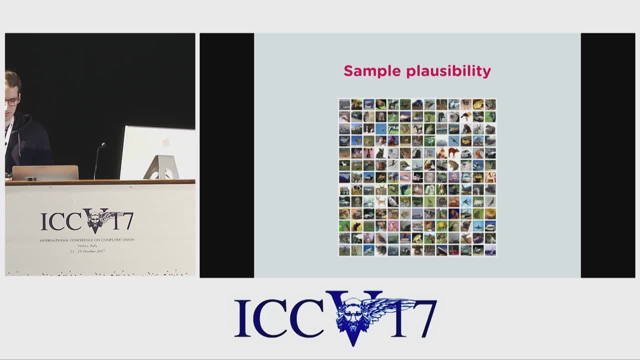 models. One heuristic which is, of course, commonly used is to look at samples and and look how plausible they are, even when we are actually not that interested in the samples themselves but are interested in something else. We've already discussed a few cases where this can go wrong, but maybe you think maybe we can detect those cases, rule them out. 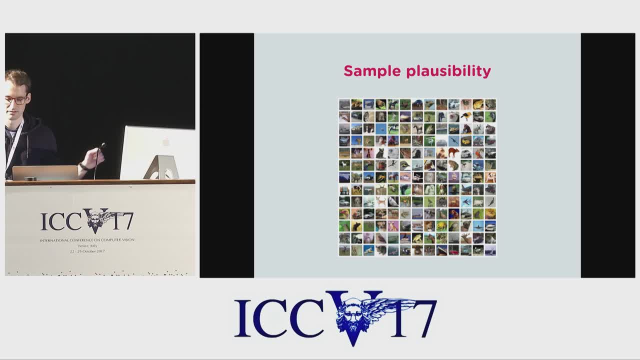 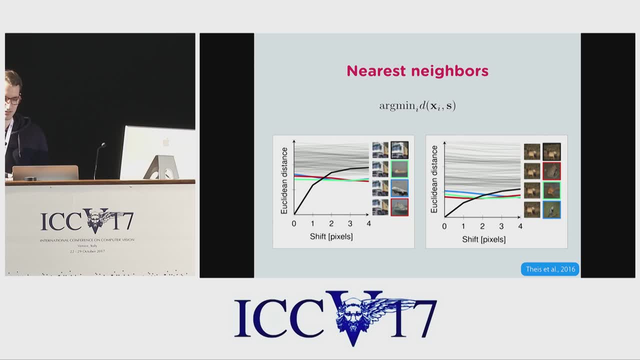 and then samples will again be informative. So, for example, a lot of people have tried to detect overfitting based on these samples, using nearest neighbors. So here the basic idea is you sample from your model and then you take those samples and look for nearest neighbors in your training set and the 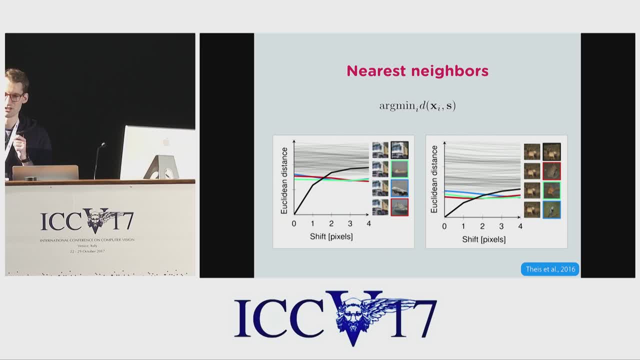 idea is that if you're training set images look very similar, suspiciously similar, to your samples, then your model has overfitted, and if they look different, then your model has not overfitted. But this has some problems. The main problem is that already 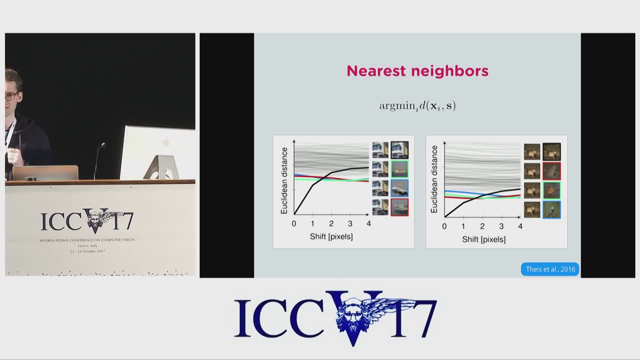 very small changes to images in the training set can lead to completely different nearest neighbors. So what we have done here is we've generated slightly shifted versions of images in the training set and here and measured them. So what we've done here is we've generated slightly shifted versions of images in the training set and here and measured them. 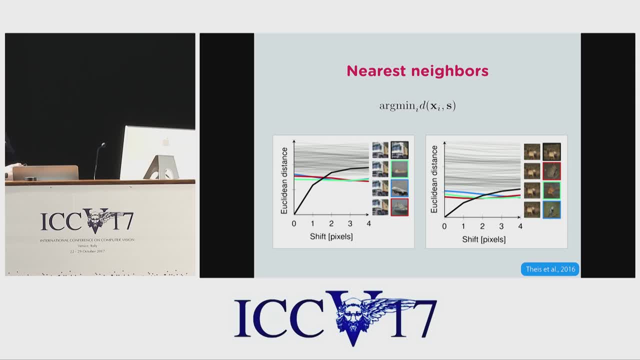 the Euclidean distance. here on the x-axis you have the shift of the number of pixels of the training image on and on the y-axis we have Euclidean distance and then each of these lines represents a Euclidean distance to an image in the training set. so each line is a represents an image in the training set. 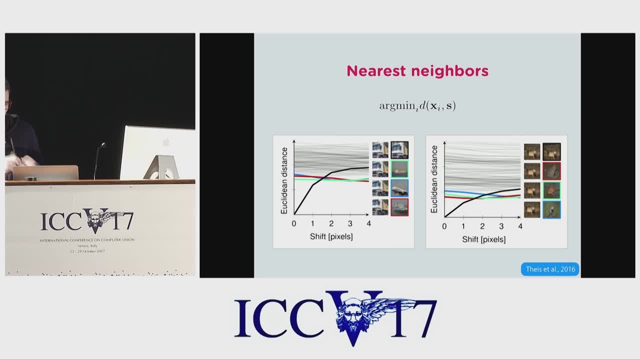 for example, the black line represents the Euclidean distance to the non shifted image, to the reference image. so, for example, of course, at a zero pixel shift the Euclidean distance will be zero. and as you shift this image the Euclidean distance will increase. and the problematic thing here is that already 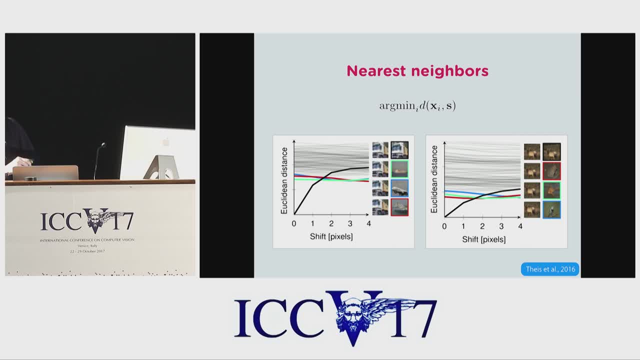 after a two pixel shift, different images in the training set become the nearest neighbor. so you can also see that here on the on the right hand side, the first column, are the differently shifted versions of this image and you can see that they almost look identical. and in the second column we have the nearest neighbors in the 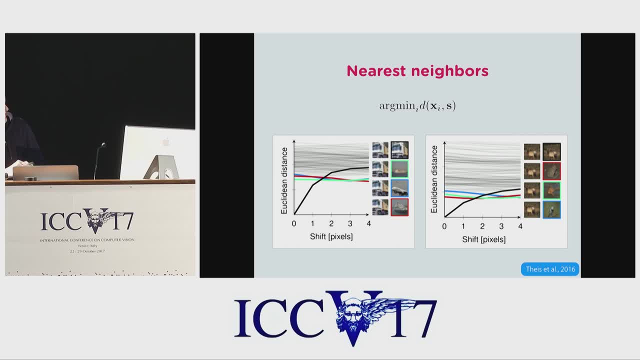 training set and, yeah, already, a two pixel shift will not only give you a slightly different track, but it will give you a completely different image. so basically what this means is that this test will only be positive if your model actually does store the training set as soon as it makes introduces. 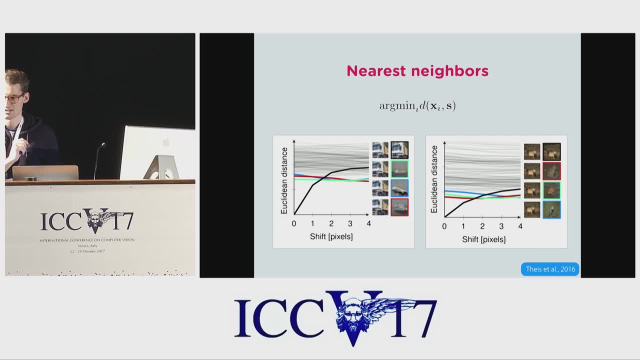 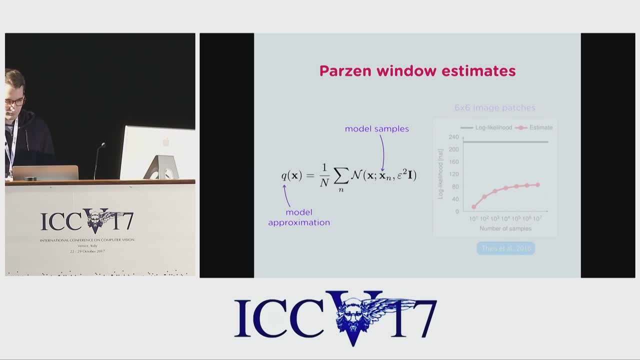 slide errors into your training images, this test will already fail and will not tell you anything. another thing that people have done is to use what's called parsnwingow estimates, and here the basic idea is: we again generate samples from our model and then we fit a another model to these samples and use the log likelihood. 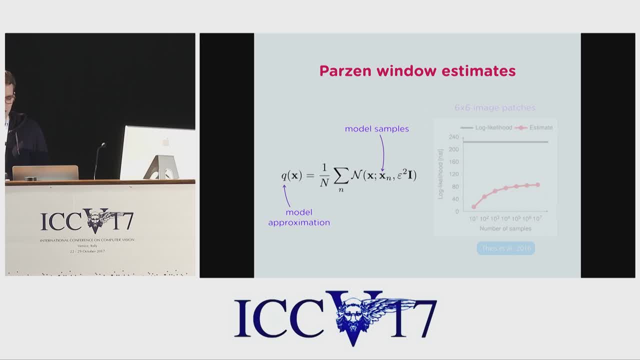 of this model as a, as a proxy for the real log likelihood of the of the underlying model. so the first problem of this approach is that the, the approximation that we get to the log likelihood, is extremely, extremely poor. to show this, we fit it in a full covariance gaussian to: 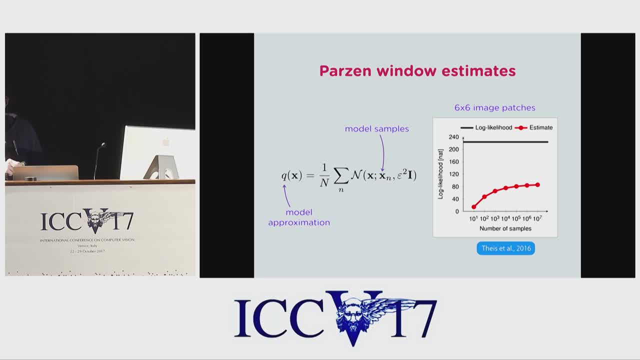 only six by six image patches. you can see the log likelihood of that gaussian here, that's the black bar, and then for various numbers of samples we get a different parsing window estimate. you can see that the estimate is extremely far away from the true log likelihood of this gaussian model. 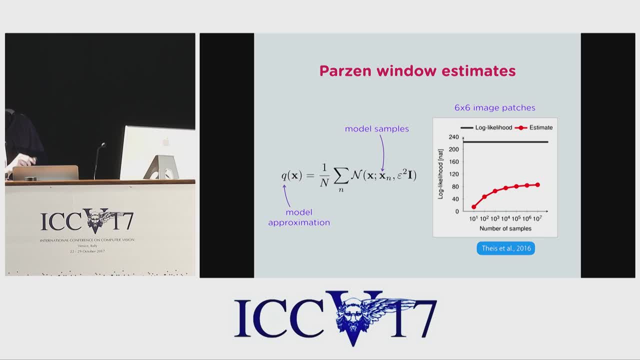 and that is despite, you know, us using a lot more samples than what is common in the literature. and that is despite us using much smaller images than what is common in the literature. and that's despite this being a very simple model. it's just a gaussian model, um, but this would all still be fine if at least the parsing window estimates. 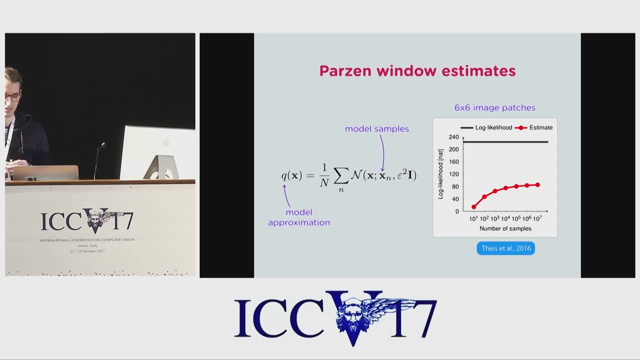 ranked our models in a in a meaningful order, right like we. if we don't actually care about the log likelihood, but we just care about the, the ranking of the different models, then that might still work, but we find that this is also not the case. instead, we find that you can get: 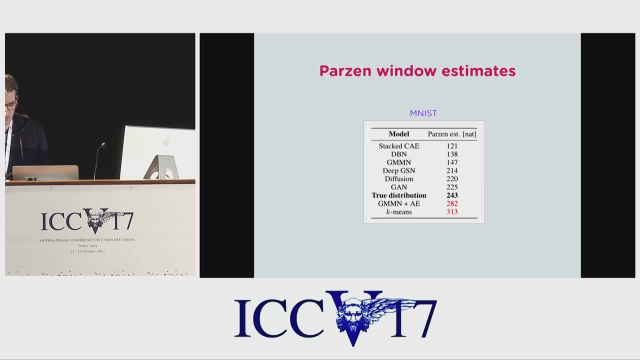 even better performance than than anything that has has been published in the literature before. so let's look at this again. we're going to go through this in a bit, but this is a very simple example of how we can get a better performance of the model by just doing k-means and then sampling. 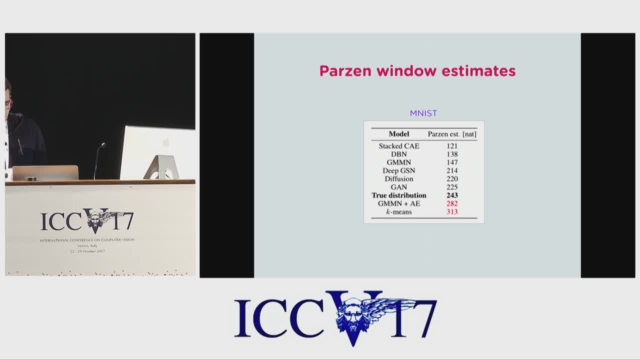 means and use and use that as your samples and that will give you a parsing window score which is better than any other published result and, even more worryingly, it's even better than the real distribution of natural images or, in this case, in amnesty. so basically what this means: 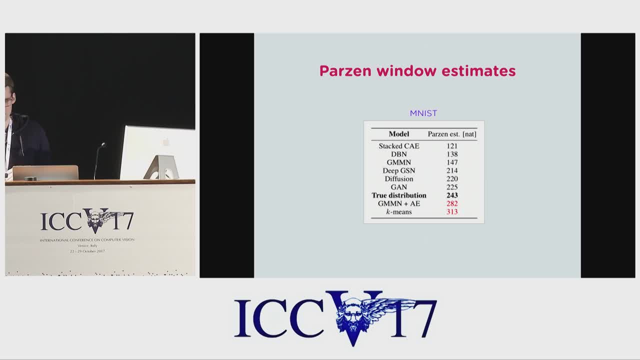 meaningful ranking of your models. It does not measure what you think it might measure and it probably should be avoided. Alright, just to summarize what we've talked about, we saw a couple of examples of how to evaluate generative models, and the point of this exercise was to show that you know meaningful 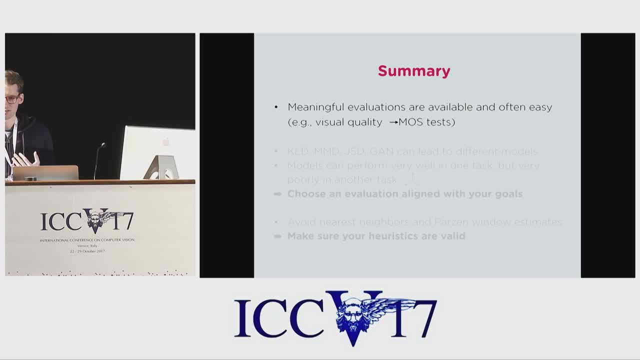 evaluations are available. if you know what the goal of your generative modeling is and why you're training a generative model in the first place- and then we saw that you know different metrics and different applications can favor very different models- Your model might perform very well with respect to 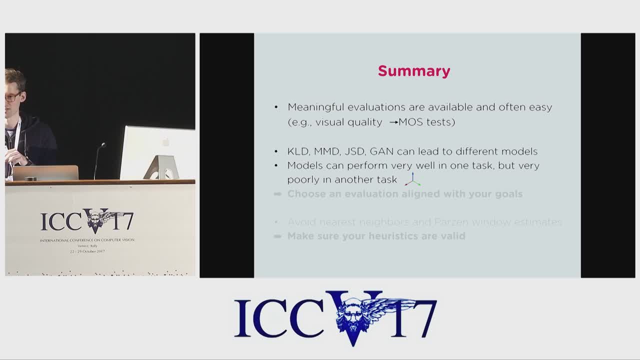 one application, but very poorly with respect to another application, and so you shouldn't draw any conclusions about the performance in one application from another application. And finally, we've looked at some heuristics for evaluating generative models and saw how they can fail, So that just means if you 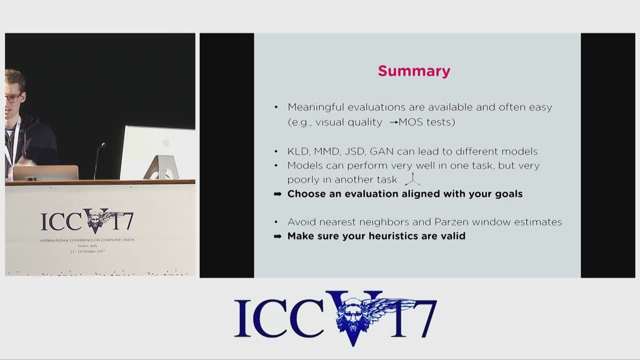 absolutely have to use heuristics to evaluate your generative model. you should make sure that they actually measure what you want them to measure, and you should probably also test that they can't be easily cheated by models which you wouldn't consider a good model. 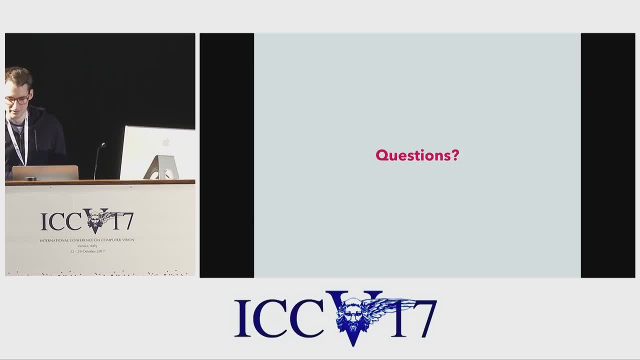 Alright, let me know if you have any questions. I'd like your example of trading sample quality for log-like data, but I wonder: how unique are those distributions? Have you selected distributions randomly from all your models? So if you actually do train generative models, for just log likelihood, let's say you do- 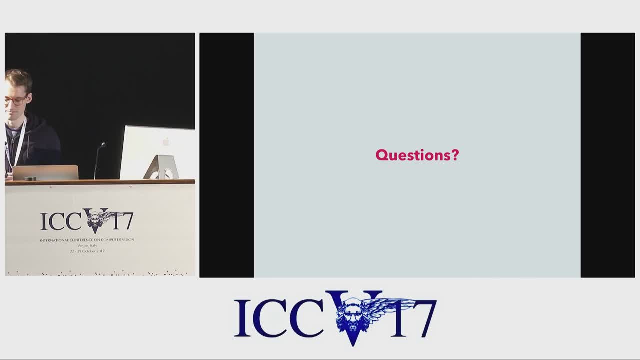 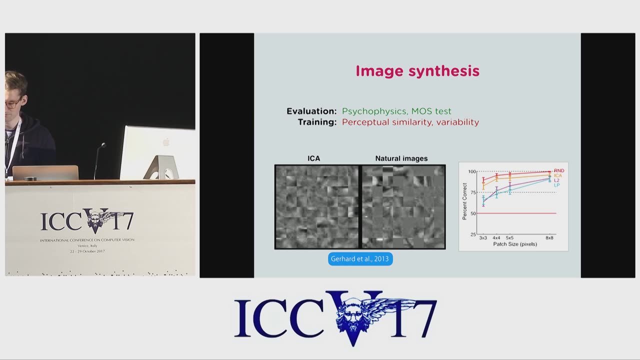 find a correlation between sample quality and log likelihood. This was shown also in this paper, where better models actually do produce better log likelihood. But that only holds true for models which are, I think, optimized for the same criterion, right Like, if you start to optimize models for different criteria, then they can have completely different. 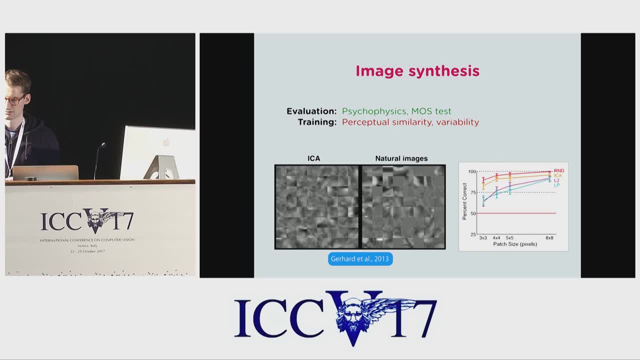 rankings. Okay, I guess people want to go to lunch. All right, fine.